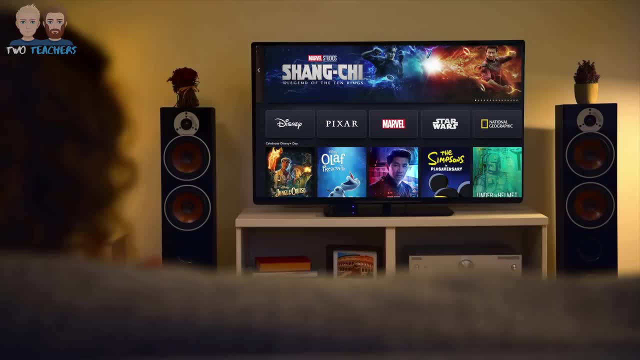 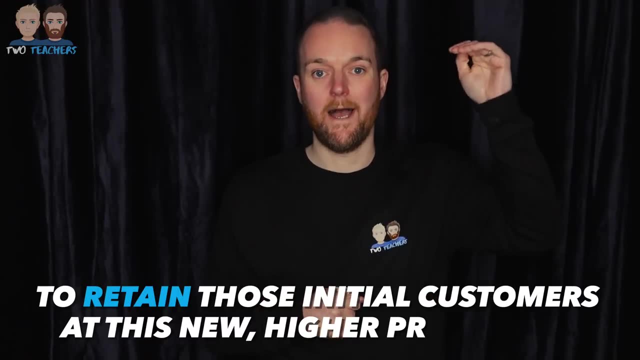 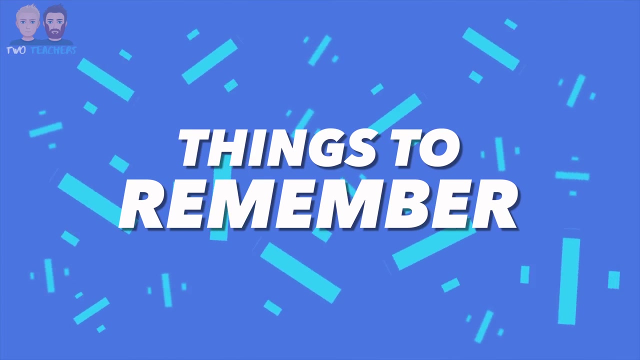 much more closely matched to those of their competitors. Disney Plus is now hoping that the quality of their content is good enough to retain those initial customers at this new higher price point. Making the business more profit per subscriber Sounds easy, but there's a few things to keep in mind when using penetration pricing. Firstly, you need to have a clear 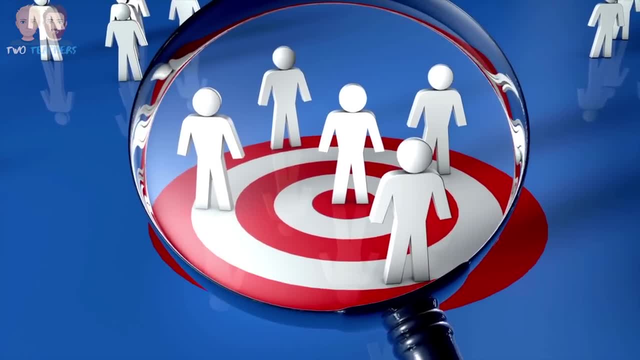 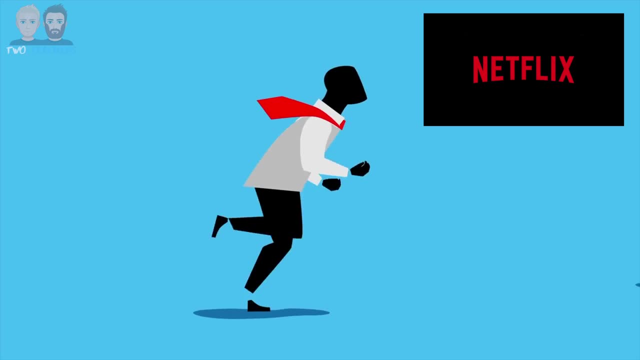 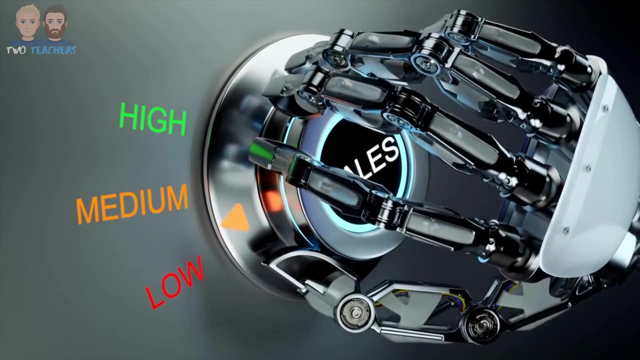 understanding of your target market and their price sensitivity. If your target market is more price sensitive, then they're likely to jump ship when you start to begin raising those prices, Making them more likely to switch to one of your competitors. Secondly, you need to have a plan in place of how you're going to eventually start raising those. prices. You don't want to be stuck in a low price trap forever and in Disney's case, they needed to provide quality content to ensure subscribers continue to subscribe once prices begin to rise, As customers still valued the service once the penetration pricing strategy had disappeared. 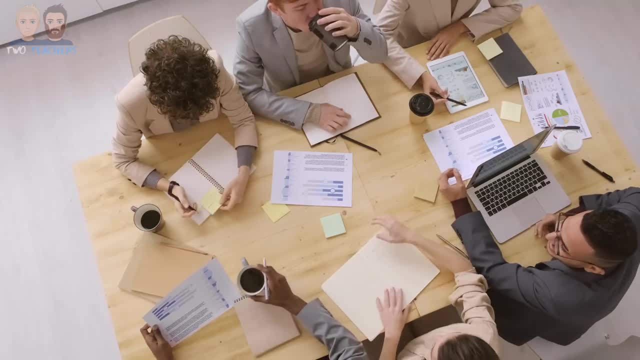 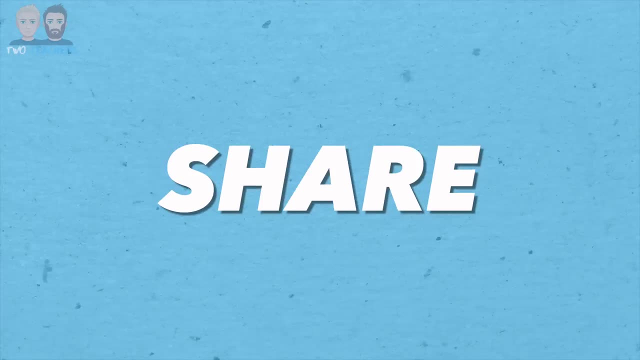 But why do companies use penetration pricing? Well, a study by Essentia found that companies using penetration pricing saw 2.5 times faster growth in market share compared to those that didn't use that pricing strategy. Another study by McKinsey & Co revealed. that penetration pricing led to 8% sales growth and 7% higher customer retention. These numbers show how powerful penetration pricing can be at helping a business gain market share and establishing a brand in such a competitive market.